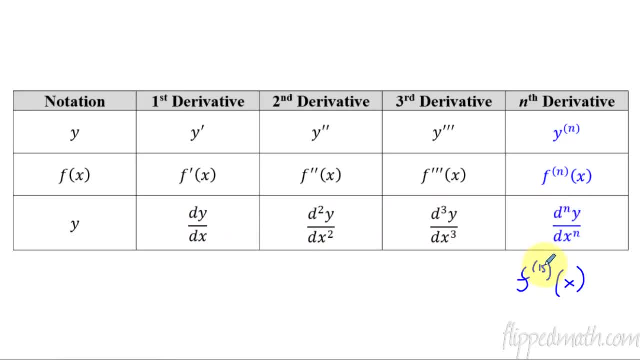 you would say d to the nth, or in other words the 15th derivative x to the 15th. So nothing really new going on here, except maybe a little bit of this notation. Just make sure you have that written down. You understand this chart here for your notation. 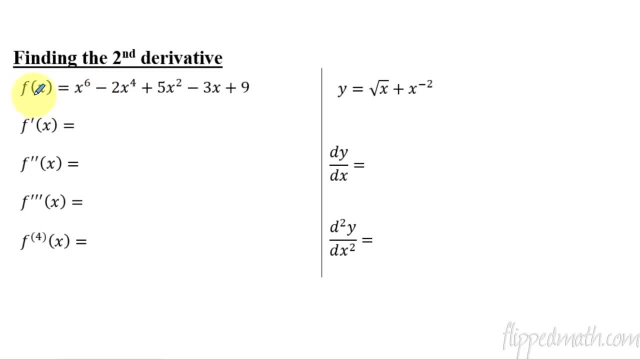 Now let's actually take the derivative. So here we have a polynomial function, And if we take the first derivative, we're just going to use the power rule here. So 6x to the 5th minus 8x, cubed plus 10x minus 3.. And then the plus 9 becomes a 0, because it's a constant. 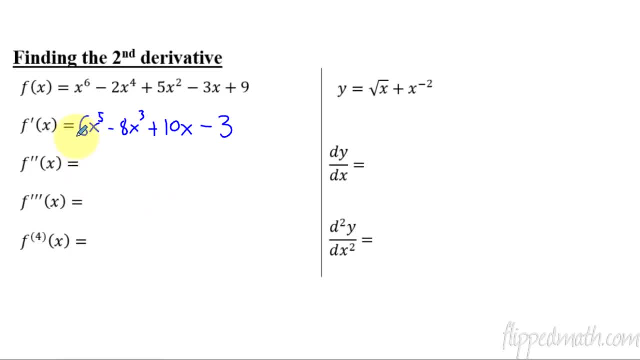 All right, so that's the first derivative. The second derivative is just taking the derivative of the first derivative. It's that simple. The derivative of the first derivative gives you the second derivative. So we'll just do the same thing again: 30x to the 4th. 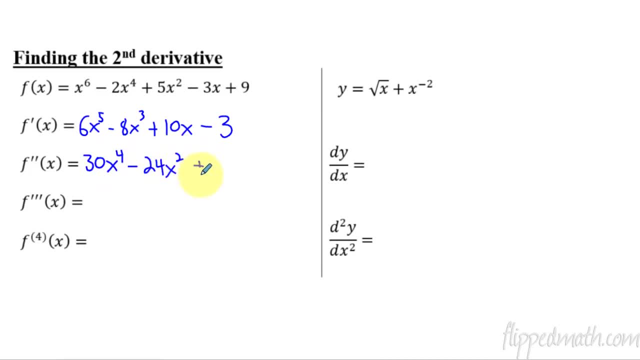 minus 24x, squared plus 10.. And the derivative of a constant is 0.. And then here let's do the third derivative. We just take the derivative of the second. So 30 times 4, 120x cubed minus 48x. 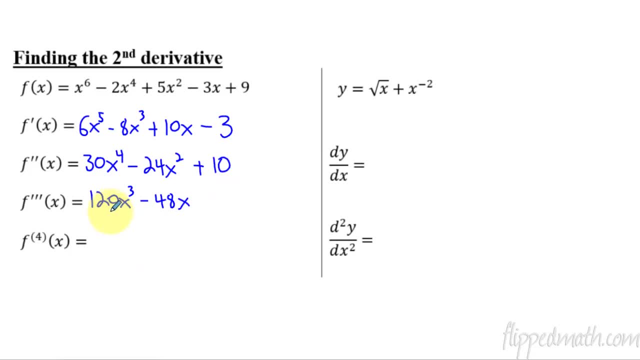 And then the derivative of 10 is just 0.. And then the fourth derivative: 120 times 360, 360x squared minus 48.. And we could keep going, The fifth derivative. this would be gone, And eventually- and this is kind of interesting- 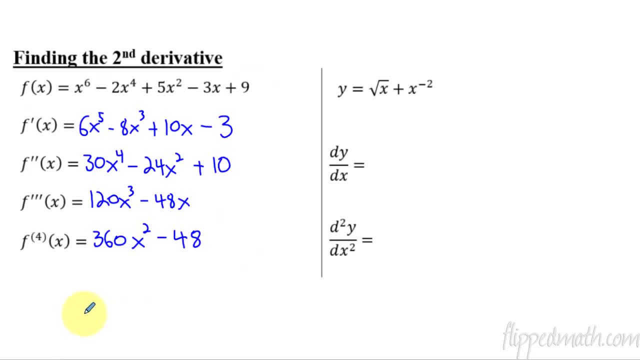 if you have a polynomial function, if you take enough derivatives, eventually you're going to end up with 0.. If you take enough derivatives, eventually you're going to end up with 0. When you finally get done, because it's going to come down to a constant. 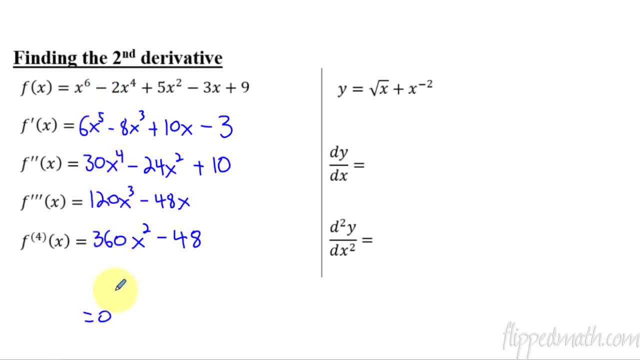 the derivative of a constant is 0. So if you just kept going, going, going, going going, you'd eventually get down to 0. But that only works if it's a polynomial function. Over here this is the same thing. We're doing the same thing, It's just I have different. 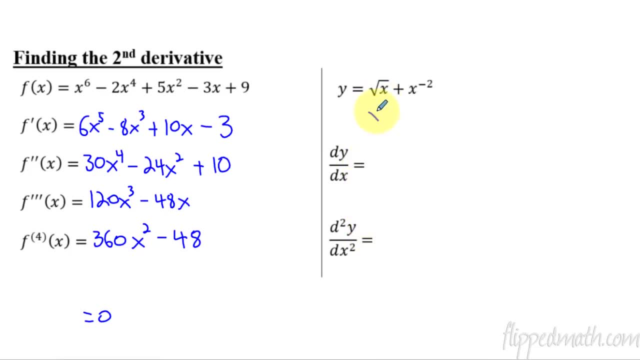 notation. I want to show you the difference. I'm going to rewrite this, though. Let's write this as x to the 1 half plus x to the negative 2. So it's a little easier to take the derivatives. So the first derivative is just 1 half, x to the negative, 1 half. 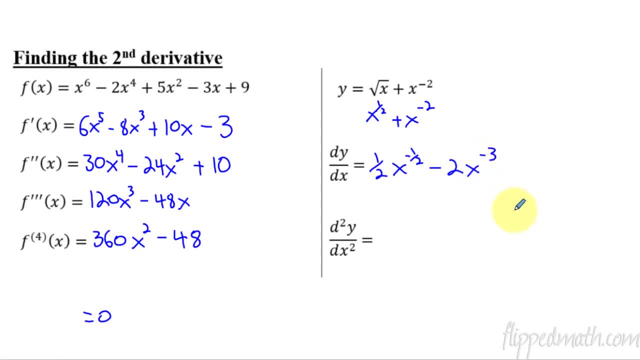 minus 2x, squared, squared. And then we're going to write this as x to the negative 3. And we could simplify that, but we wouldn't want to. yet We wouldn't want to rewrite this because we're trying to take its second derivative. So now we use the power rule again, So we get negative 1, fourth x. 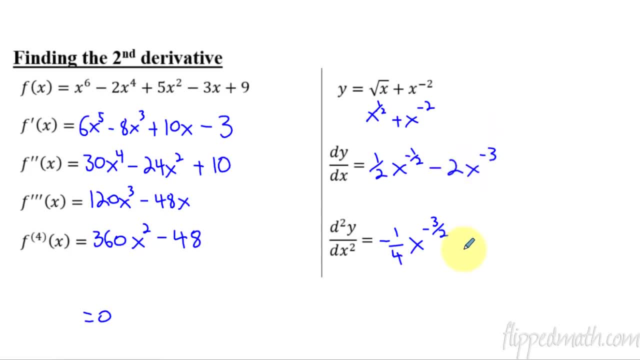 to the subtract 1. We get negative 3 halves, And then here the negative 3 times negative 2 is plus 6 x to the negative 4. And then we could rewrite that one if we wanted, But that would be the second derivative. 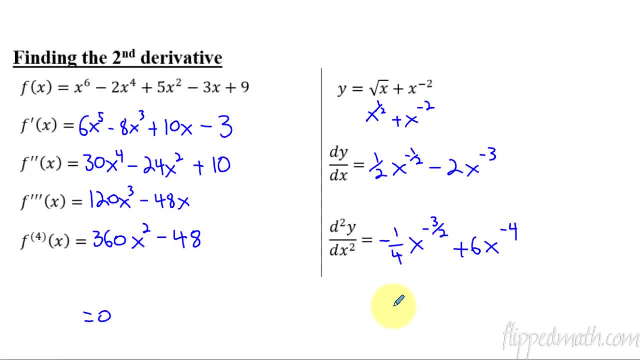 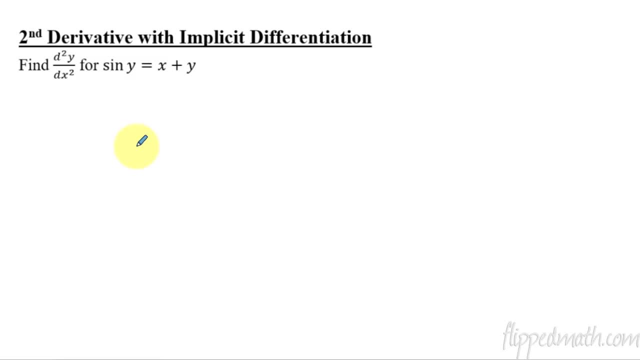 OK, So nothing really earth-shattering new or tricky, Literally taking the next derivative. That's how you do this. This is the tricky part: Implicit differentiation. I'm only going to show you one example on this, because it kind of repeats itself over and over. 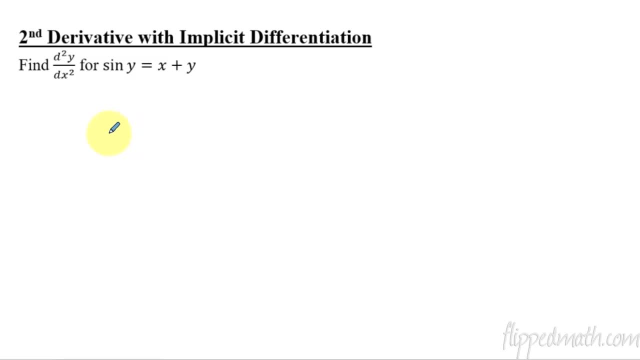 again how you do the derivative with implicit differentiation. Second derivative. I should say So just really pay attention how we do this. All right, So in order to find the second derivative, we first have to find the first derivative. So derivative of sine is going to be cosine y And then times the derivative of the inside. 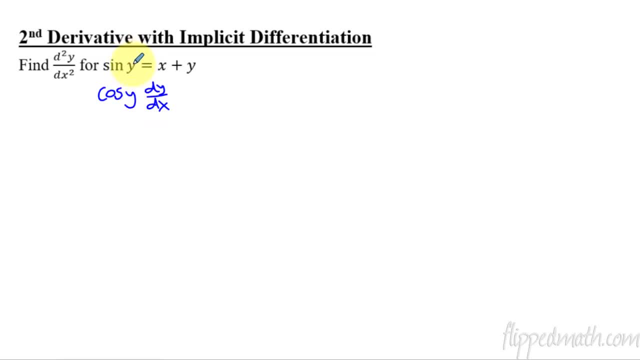 gives us dy dx. So remember, if you're ever taking the derivative of the derivative, of the derivative you're of y, you also have to include a dy dx. okay, and then equals: the derivative of x is 1 plus the derivative of y is 1, and then times dy dx. all right, let's get the dy dx is on the same side. 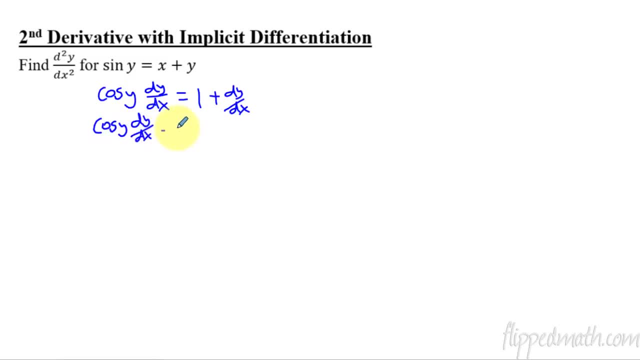 so cosine y, dy dx minus dy dx- let's make sure that's clearly a minus sign- equals 1, factor out at dy dx. so remember this from a few lessons ago: I hope: cosine y minus 1 equals 1 and then I finally have that the dy dx is going to equal 1 over cosine y minus 1. okay, so now we'll take the. 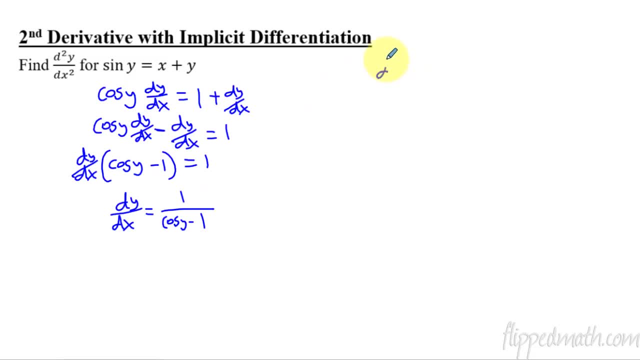 second derivative. so I'm going to come back up here and start over again. I'm going to say that the second derivative, so d squared, y over dx squared, is going to equal the derivative of this. I want you to rewrite this as cosine y minus 1, raised to the negative 1. that makes this a little easier, if you can. 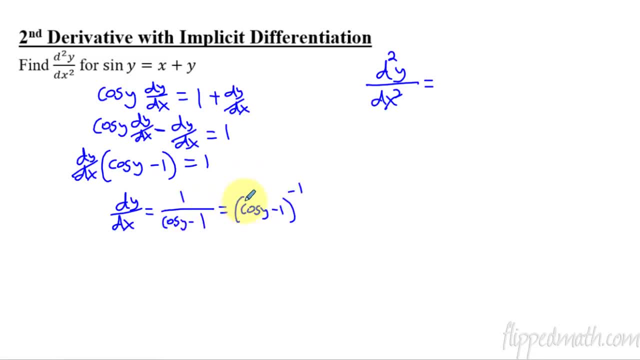 think of this. as this is all raised to the negative 1, then you can just see it's going to be the chain rule. okay, so let's apply the chain rule here. this is negative, 1 comes down to the front and then it's going to be cosine y minus 1. 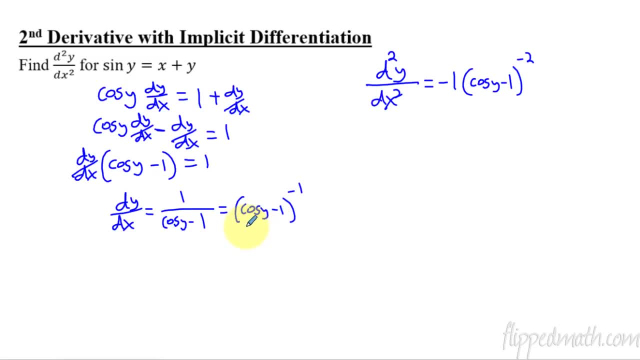 and now it's raised to the negative 2 times the derivative of the inside. now we got to go the inside and tapes the derivative of that. so the derivative of that is going to be negative sine y. derivative of negative 1 is just 0 times. 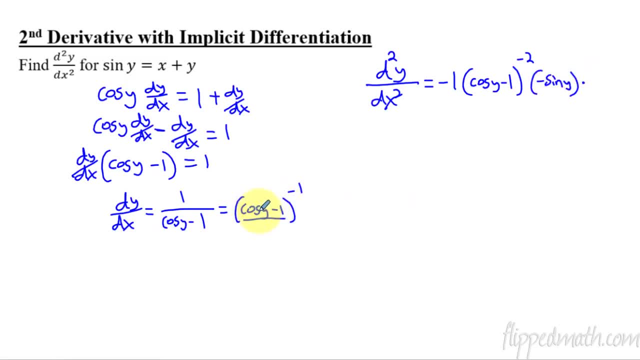 the derivative of. we got to go. we did the derivative of cosine y. now you have to do the derivative of y, which is dy dx. okay, this is where it becomes a little bit more complicated. in fact, I'm gonna do this d squared y. let's clean this up. 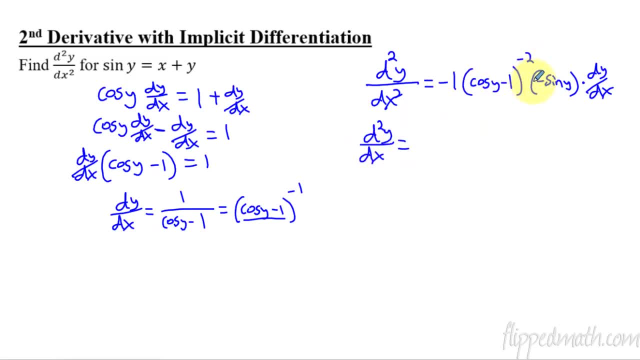 just a little bit before we do our next step. so the negative and the negative, those just cancel, and so I'm going to have a sine y on top of a fraction. on bottom I have cosine y minus 1 quantity squared, and then I have times dy dx. so 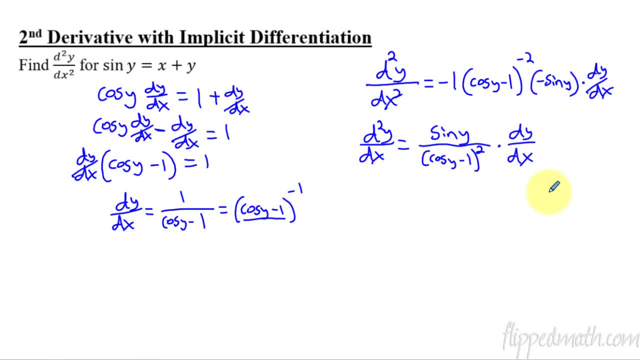 now it is literally. this is how all of these problems work for implicit differentiation. you always end up with a dy dx here in your second derivative, and when that happens, what do you do with it? you, that's where you do substitution. we know what dy dx equals. it equals this, so that 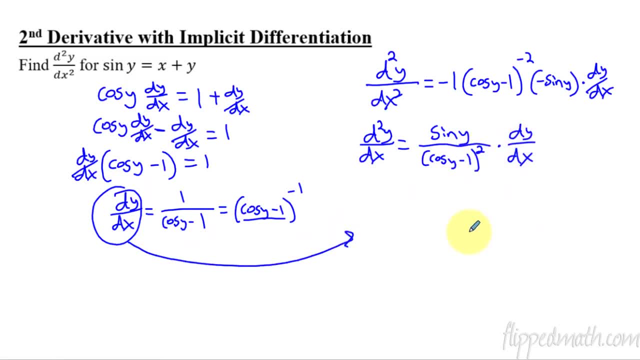 dy dx goes over here to that dy dx. so we are literally just substituting in this whole thing right there. so this becomes sine y over cosine y minus 1 quantity squared times, and then it's dy dx. we substitute in what it equals, which is just 1 over. 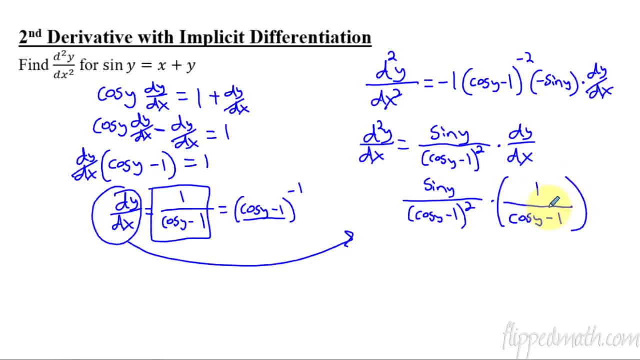 cosine y minus 1, that's dy dx, and then you're done. yeah well, I mean, simplify sine y over, and then we have a cosine y minus 1 quantity cubed now, since there's three of them, and so that is the second derivative with implicit differentiation. oh, I forgot little. 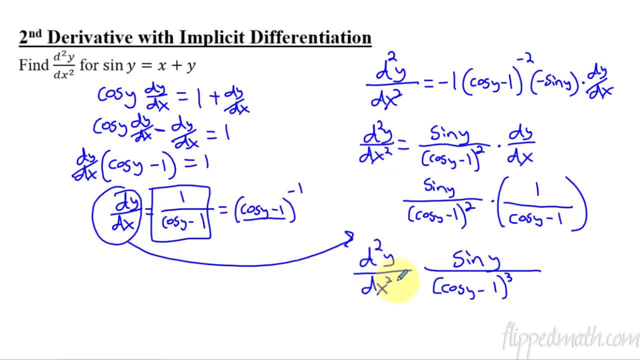 squared right there. sorry, squared dx squared. so that's the second derivative, implicit differentiation. it's all about substitution. once you get a dy dx, you have to go back to the previous step of what was dy dx. now in this packet, in this lesson, there'll be a couple other little things that get thrown out at you that make you think about derivatives and 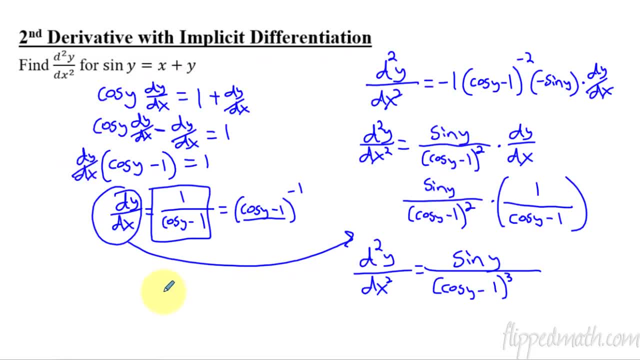 second derivatives and all that, but this is the gist of what you have to work with, so rock that mastery check and the test. this is the last lesson for unit three and i'll see you back in our next unit.